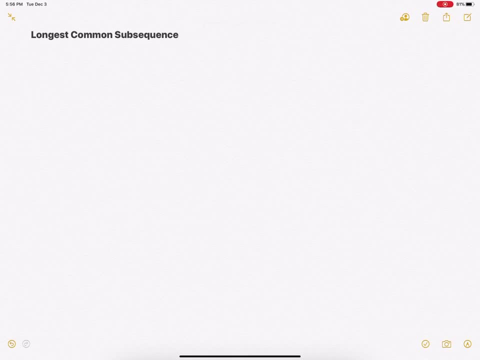 Hi everyone. in this video we'll study longest common subsequence. Longest common subsequence is an important problem in algorithms and it's a very important interview question as well. So let's first try to understand this problem. So for this, we'll consider character strings. 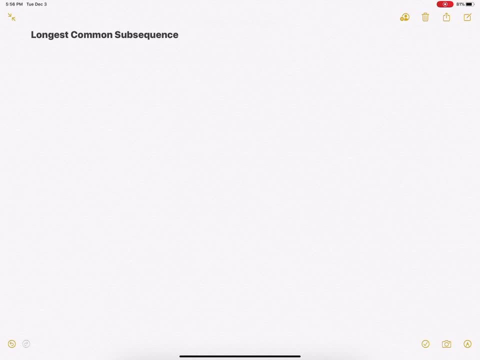 as a sequence of characters. So we can consider that we have two strings, x and z. So these are two strings or a sequence of characters. Now let x be abracadabra. This is the string x. Now let us consider another string named z, which is ada. Now z is a. 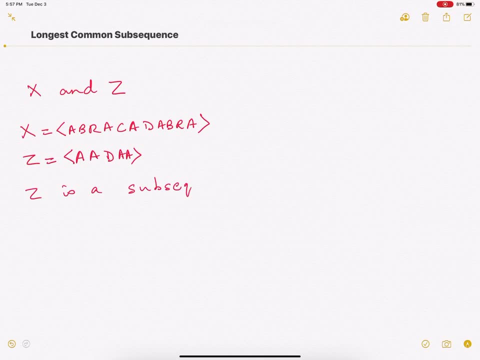 subset. This is a sequence of x. Now, why is this the case? Now you see a. if you consider the a in z, there is an a in x. Now, if you consider the second a in z, you can move ahead and you can see that. 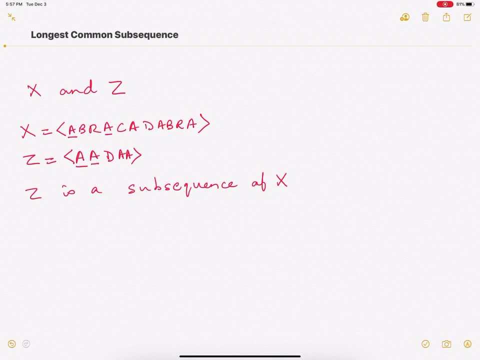 you could consider this a. If you consider this d, move ahead. You consider this d, consider this a, Consider this one, Consider the last a. So these five characters form the subsequence. So in the subsequence, you can only move continuously in one direction. You can't move back and forth. It's not. 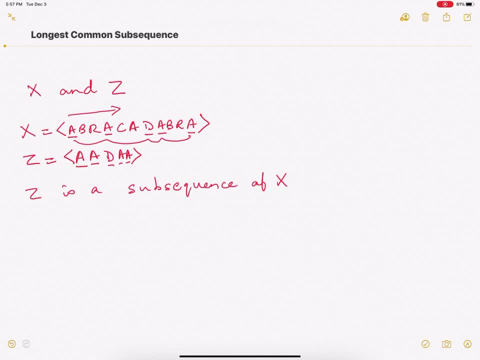 like whether these five characters are present in x. That's not the case with the subsequence. These five characters must occur in x, but they and they should occur only in that one direction, So all the way from left to the right. Another thing that you would have noticed is they need not be. 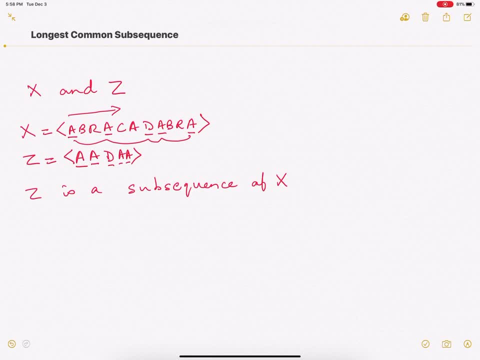 contiguous. So this is the. there's an a, then we have excluded the br, then we have picked the next a, so on and so forth. Okay, so this is what is called a subsequence of another string. So z is a. 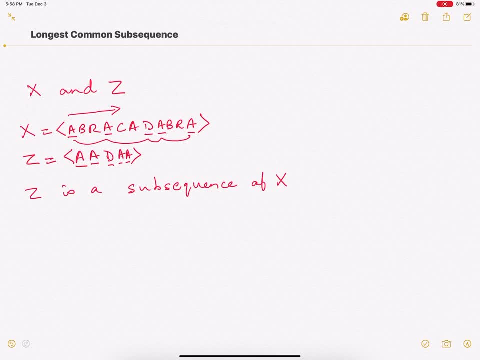 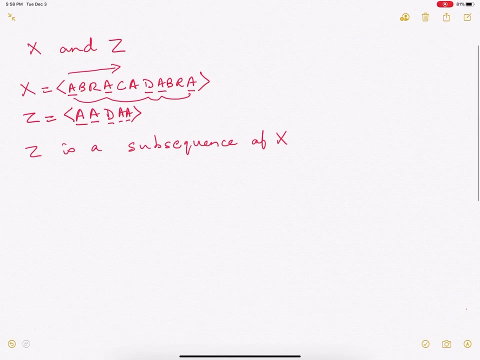 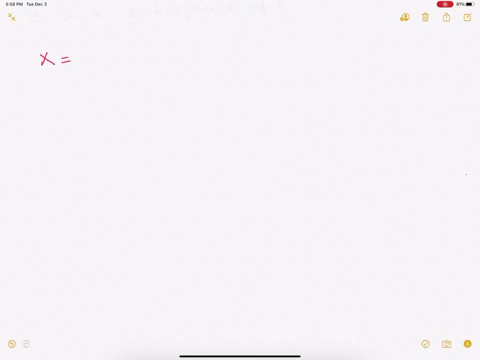 again. So x here is abracadabra. So this is what is x. Let's consider y, which is yabba-dabba-doo. So these are two strings, x and y. Okay, so there are two sequences of characters. 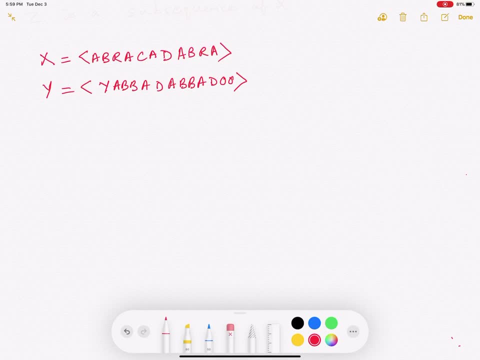 Now, between x and y, there are a bunch of common subsequences, Okay. for example, ab, a, a, b, a. This is one subsequence, one common subsequence, Okay, so this is one common subsequence. We can try and see if there are other common subsequences. 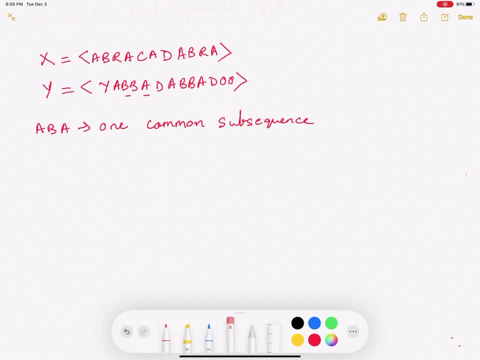 This, let me just erase this. So a a d b We can consider a a d b. So a a d b is another common subsequence. So you can find a whole bunch of common subsequences between. 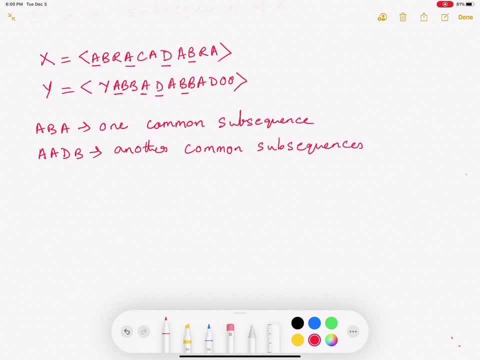 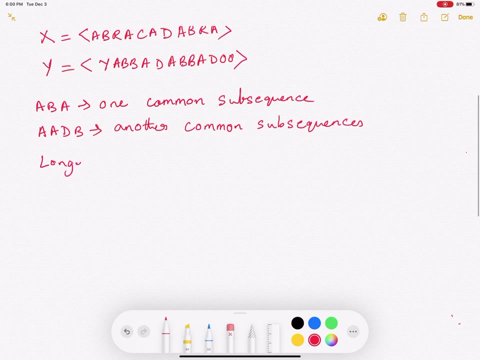 x and y here. So let me just erase this. So there are a whole bunch of common subsequences. Now our goal is: what is the maximum common subsequence or the longest common subsequence? So longest common subsequence, That's what we are first interested in between x and y. 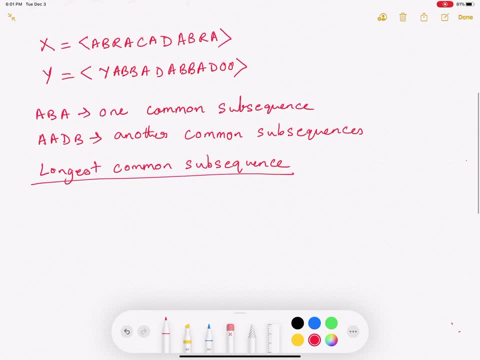 Now, if you consider x and y and if you try to find out the longest common subsequence, that will be z, which is a, b a, d a, b a. This is the longest common subsequence between x and y. So let's see if that's the case. if such subsequence exists- a, b a. 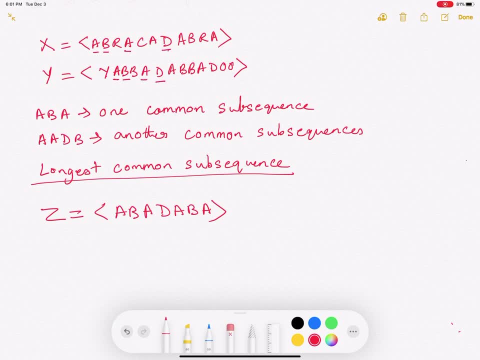 take this a d, take this d a a, take this b, this b, this a, this a, So z is the longest common subsequence. So the problem that we are going to study here is how to find the longest common subsequence. 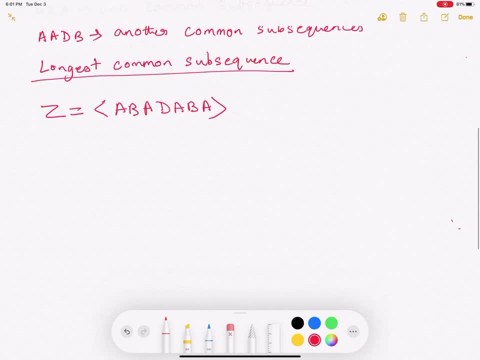 So that is the problem: b civil game fighting, b civil game fighting the longest common subsequence between two strings, two strings: x and y. okay, That's. 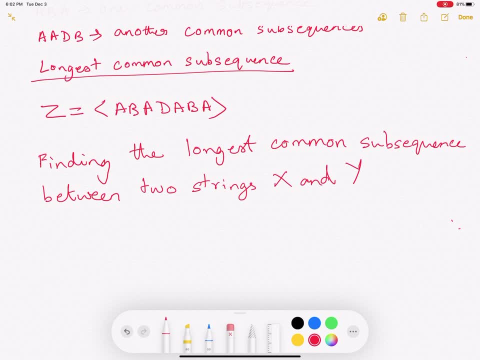 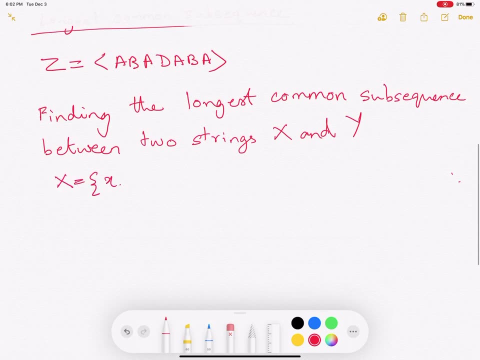 what we know Now, x and y need not be of the same length, okay. So x could be, x can be of size m, that is, x1, x2, xm. So these are all the characters in that string of x and y could. 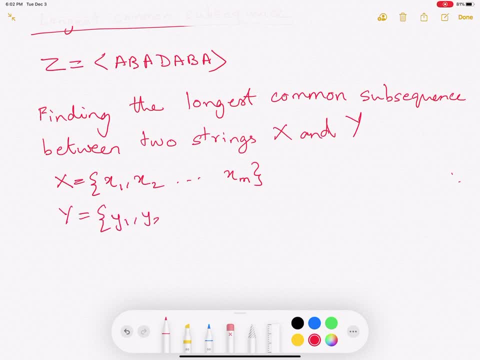 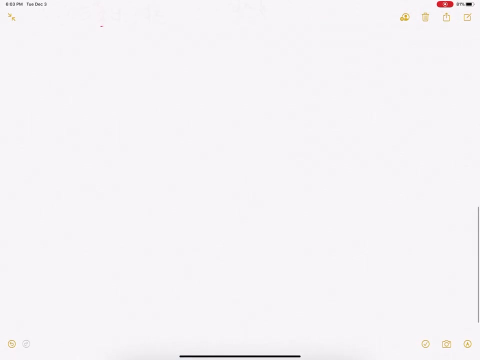 be of size n, that is, y1,, y2, all the way up to yn. So between these two strings we have to find the longest common subsequence. okay, So how do we go about solving this? Sorry about that. So we will use dynamic programming. So dynamic programming is our. 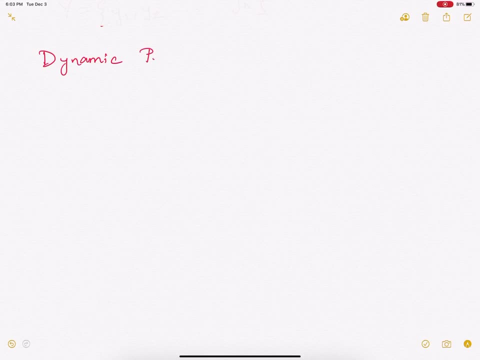 solution. If you're looking at this video, I'll assume that you have some idea of dynamic programming. I would go over this problem using dynamic programming, but I will assume that you have some basic idea of dynamic programming. If not, there is another video in this playlist which you 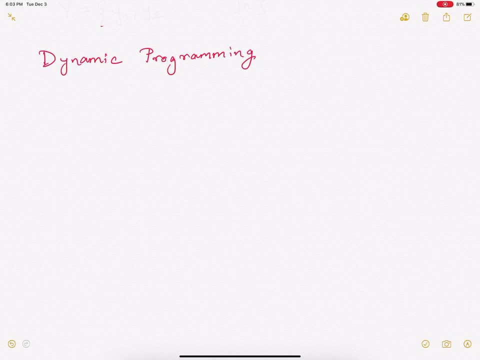 can look at to study dynamic programming. Okay, so in dynamic programming, basically what you have is we have to find out. we keep track of the longest common subsequence in a table. okay, So we'll do it in the table, And we have to first come up with rules to figure out how to fill this table. okay, So that is what we are going to do. 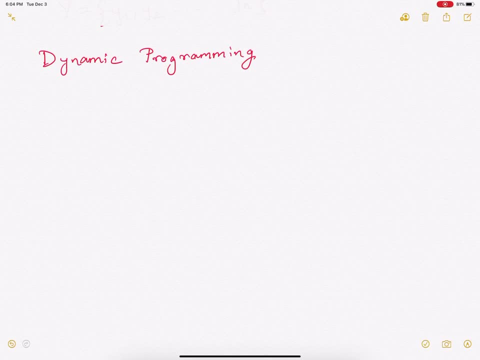 So, to understand that, let us first consider the two strings. okay, So let x equals BACDB and let y equals BDCB. Okay, So the longest common subsequence is going to be BCB. Now, in dynamic programming, what you do is: 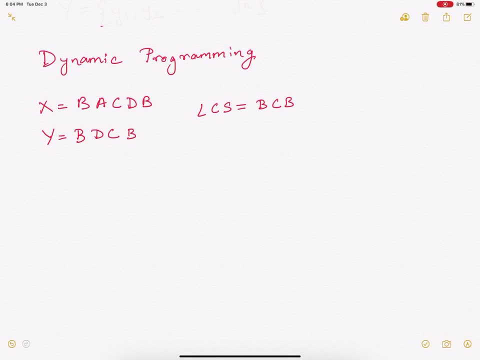 you build the solution slowly from scratch- That's what you end up doing- And you store the result in a table- okay, So what does the table contain? Okay, So let us first understand the table. So we'll have a table like this, okay, On one side of the table. 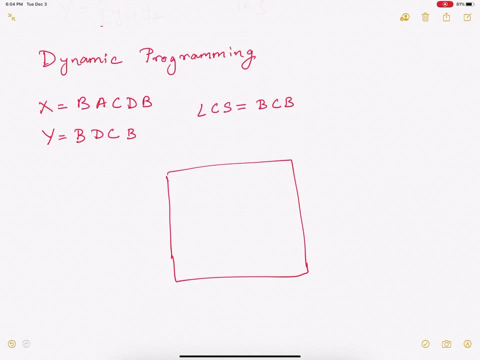 you will have this, So I'm just going to have one, two, three, So BACDB. this is what I'm going to write on this side, And on this side, I'm going to write BDCB. okay, That's what I'm going to write Now. 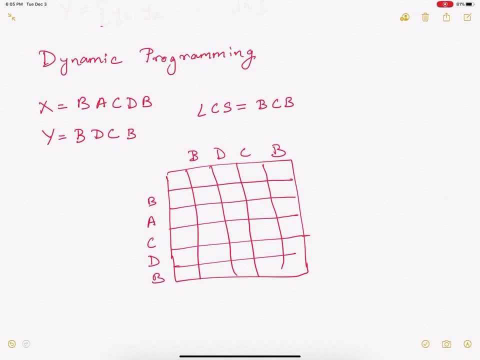 this is these are the two strings And essentially this is string x, which is of size m. So this is 1,, 0,, 1,, 2,, 3,, 4, and 5.. This is 0,, 1,, 2,, 3, and 4.. So we have a string of size 5 along one axis and a string of size 4 along this other axis. 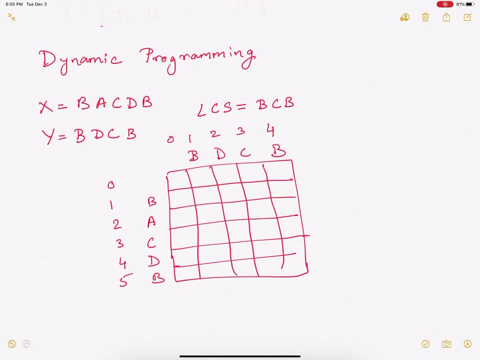 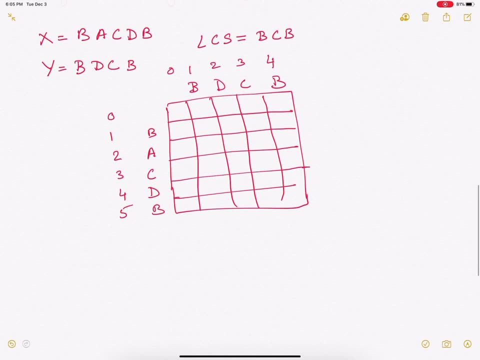 Now, what do we get from this table? Okay, So let us assume that an entry in this table is denoted by CIG. So CIG is the entry in the i-th row and j-th column. okay, Okay, It's an entry in the i-th row and j-th column Of this. 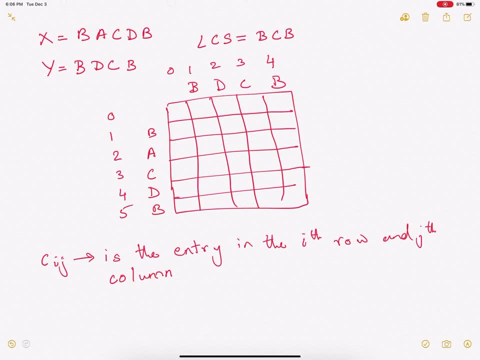 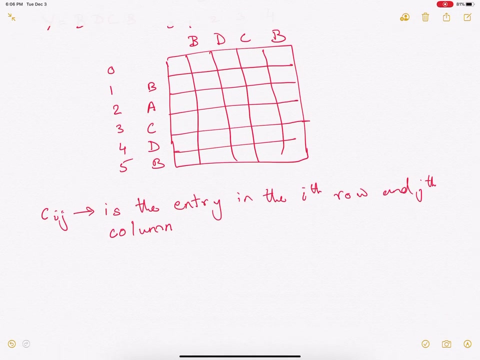 this is a table out here. Now, what will CIG store? Okay, What does CIG stand for? That's the thing that we are going to study. Okay, Now CIG captures the longest common or the length of the longest common subsequence between the two strings xi and xj. okay, 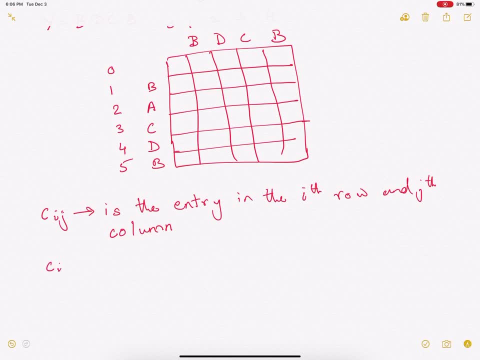 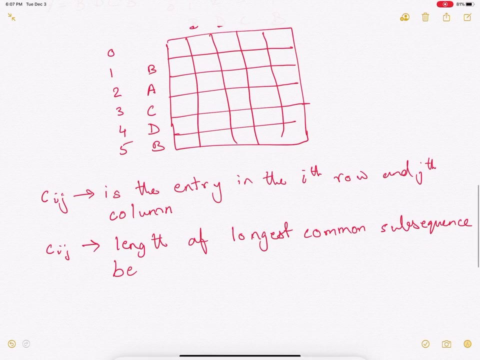 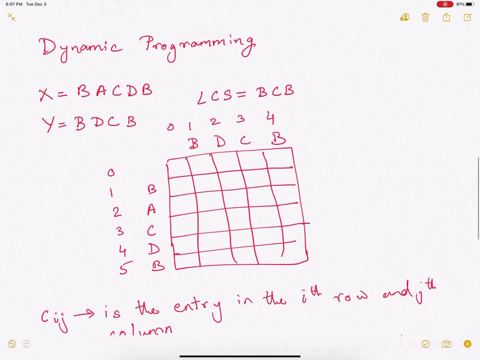 So let me explain. that captures the length of longest common subsequence between x? i and x j and y j, between x? i and y j. so so x is this one, here there is y, and what is x? i and y j? so let us assume 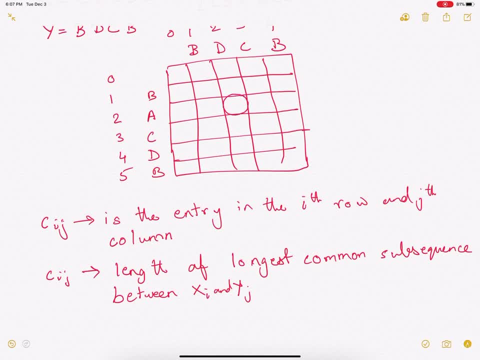 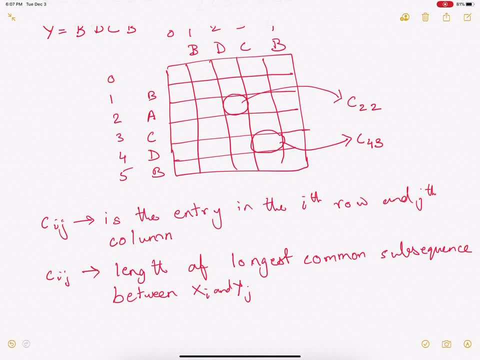 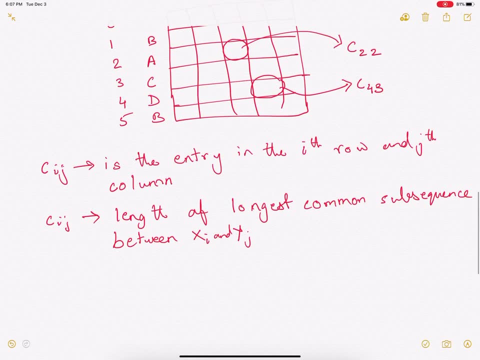 third column: okay, so. so that's what this is now. what does c43 stand for now? so in in c43, you are finding the longest common subsegment, x4 and y3. that's what you are trying to find now. what is this x4 and what is this y3? we have just so far. we've just talked about x and y, so 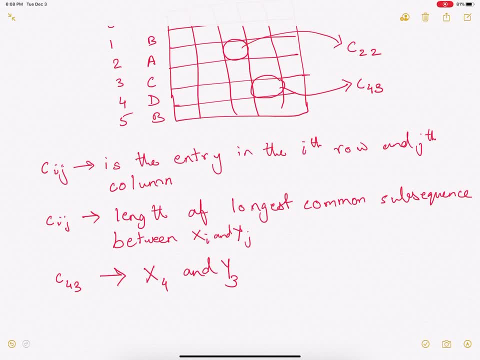 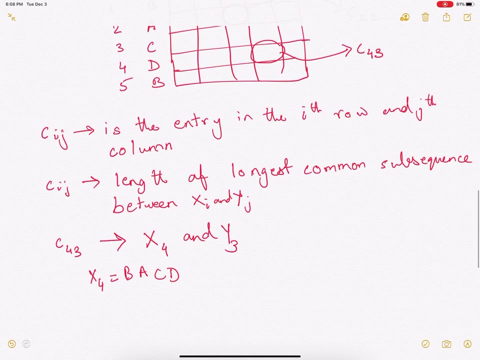 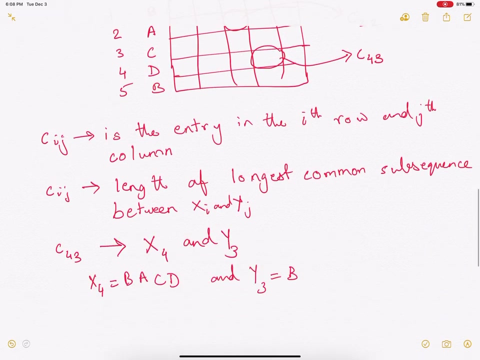 what is this? x4 and y3? so x4 is essentially the string till the fourth character. so x4 is b, a, c, d out here, and y3 is b, d, c, dc. so that's what y3 is. so what we are trying to do is we are trying to find out the longest. 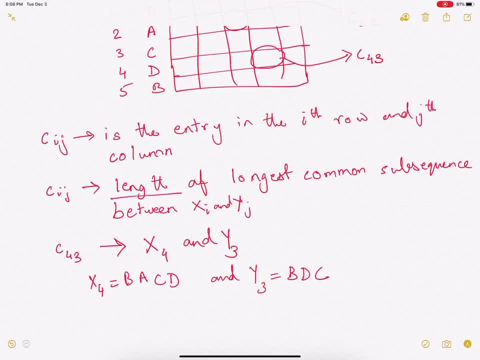 common length of a bound, so f of x and f of y, which is the longest common subsegment: x4, and y3 and x4. so that's what y3 is. so what we are trying to do is we are trying to find out the of the longest common subsequence. that's what we are trying to find out between x4 and y4. so 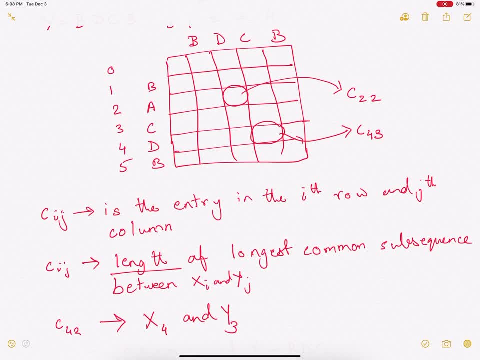 if we go back to this table, when we reach this place out here, this should give us the longest common subsequence, this entry. c54 should give us the lcs of x and y. okay, so that's what c54 that. so this is the important bit here. that's what c54 will give us, okay, so now the goal is when. 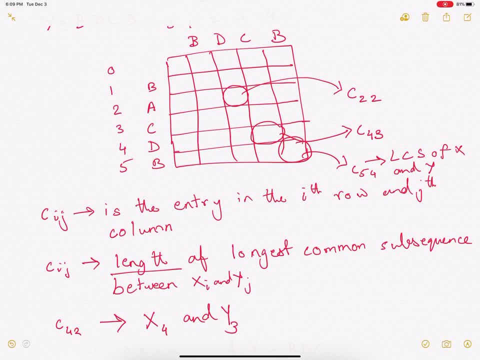 you have a table like this in dynamic programming is to first fill out the values that you know. that is called initialization. okay, so fill out. we'll start with initialization. that will be the first step, so i'm just going to write it. so first step is initialization. 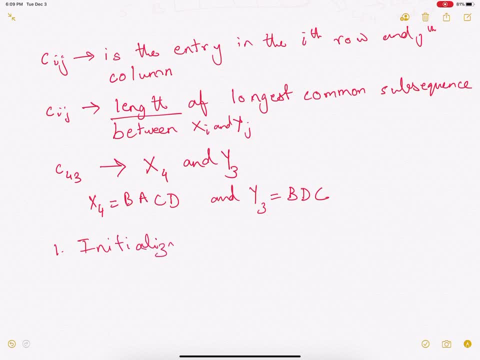 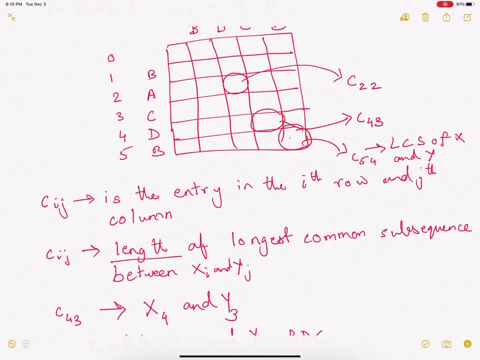 so first you initialize it, then you will have some rules to fill the table- okay, rules to fill the table- and then you will go ahead and fill the table and hopefully, when you get to the very end here, this point here, or this block, here, you will find the longest common, the length of the longest. 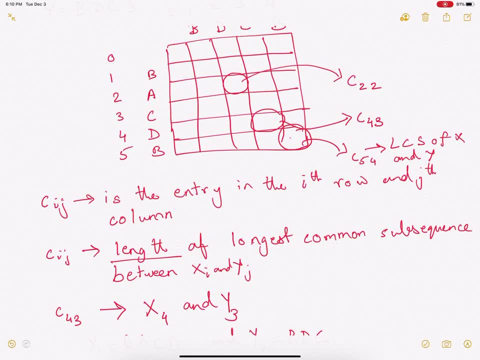 common subsequence. okay, at this point you might be wondering that if this table gives us the longest common subsequence, then you will have some rules to fill the table. okay, rules to fill the length of the longest common subsequence. how can we find the longest common subsequence? 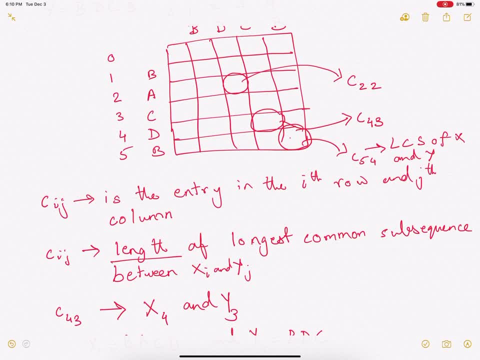 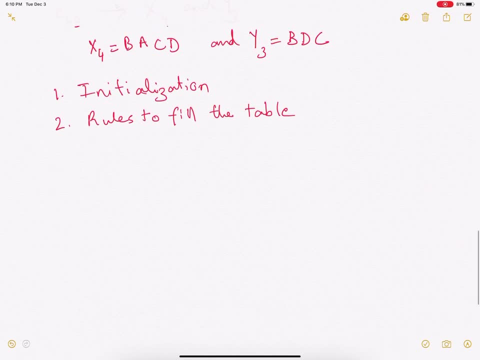 we'll get to that in a bit, but first let's try to understand what this table is going to to do. okay, so at this stage let's first draw the table again so that we can try to fill it. okay, so this table, once again, is easy. we just draw it real quick. 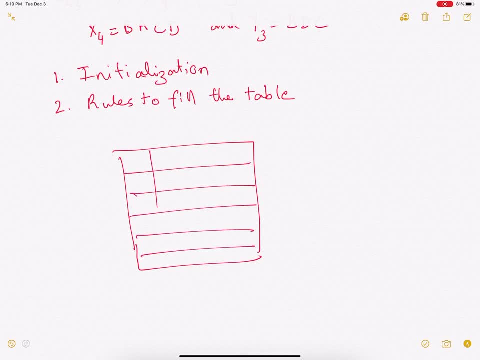 alright, do you think that you can do that? because, okay, we're about to name this table. yes, okay, so we're now going to make sure that we have something to write on this table. okay, as you can see, the label, the the bycd table, is very kort and today we know that we're going to be. 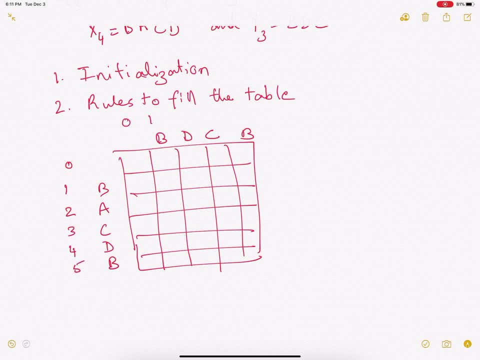 going to say, for example, copy and copy thing. we're going to say, you know, we're going to say copy and it'll give us one of these things because it's called copy, and that'll gonna begin. as an example could be type: ok, if we have like this, then we should do this type type of folder. and after the Comedy庄. 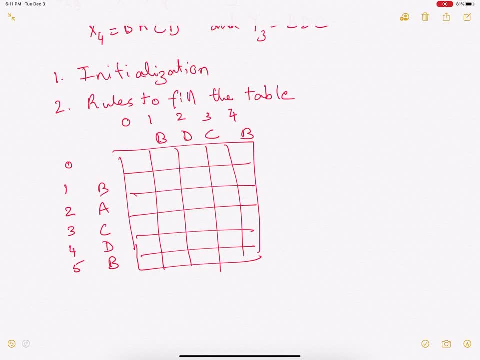 So you know two things: that c i 0 is 0 and c j 0 is 0, okay, Basically, the i-th row and the j-th column are both 0. So i-th, so when the column is 0, you just go. 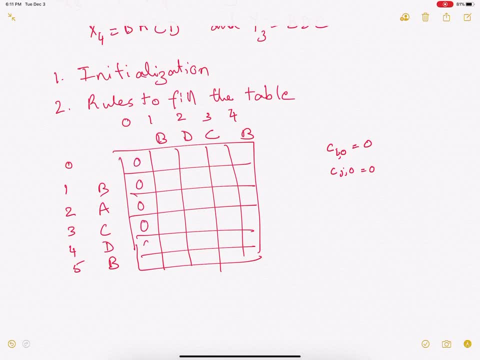 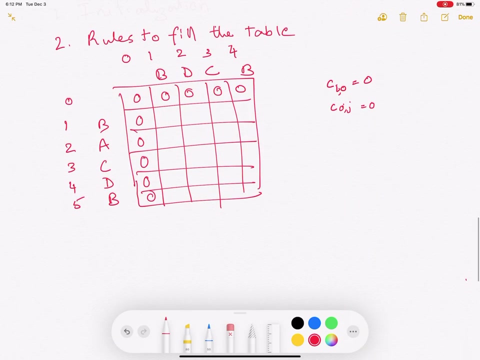 So you'll have 0s here and you will have 0s here. So this is it should be. should be 0s. okay, So that's what we know Now. Now we have to fill this. 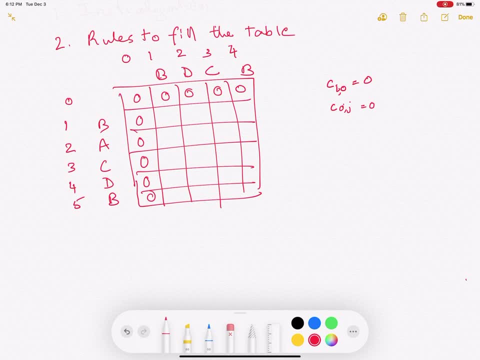 So this is the basic you start off with by filling what you know. Now, how do we fill the rest of the table Now? this is the interesting case. Now to understand that, once you've initialized, we have to consider two cases. 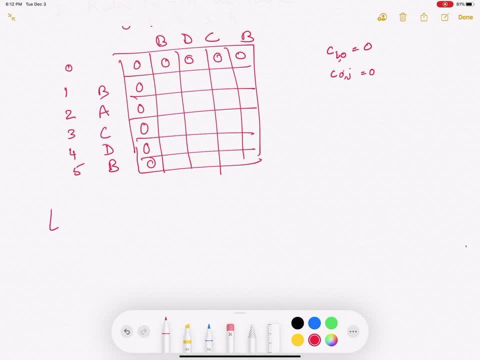 The first case is the last characters match. So let us look at this circle here. Now, when we're trying to fill that circle we have, we're considering the string BAC and BDC. okay, And so we're basically considering x3, that is BAC, and y3, which is BDC. 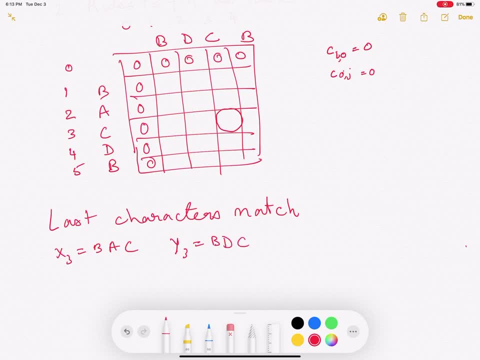 Of course we can't just start off by filling that space, but let's just consider it to understand this Now. in this case the last characters match, okay, So basically the C and C match here. Now, when C and C match, or the last characters match in the general case for Cij. 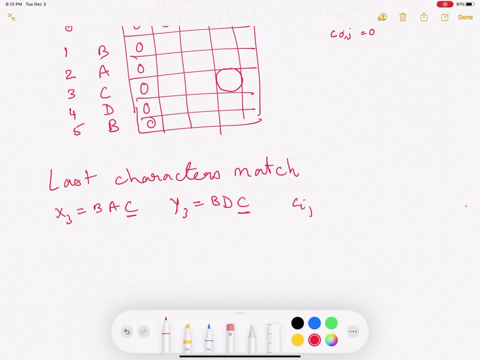 that is for Cij. if the last character, xi, equals yj- This will be the general case- Then what we can say for sure is this character will definitely be part of the longest common subsequence. okay, So this character will definitely be a part. 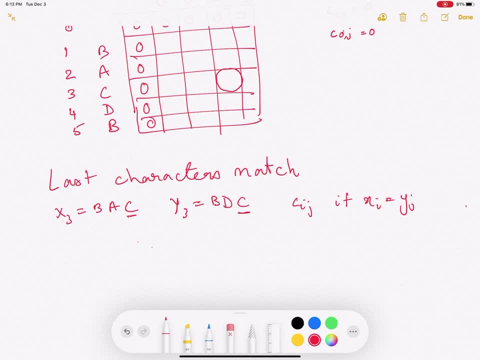 If there was another C preceding this. say, in this y, in the y, there was some C preceding this. whether you include that C or this C does not matter. So this C will definitely be a part of the longest common subsequence. okay. 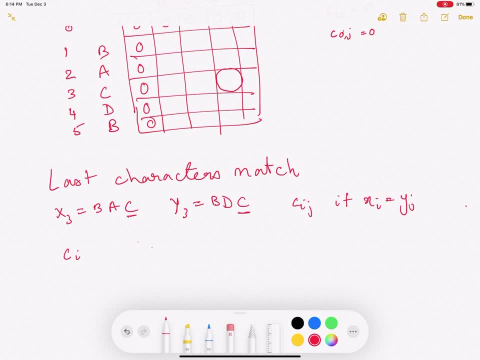 So Cij the length for the i-th, i-th, rho and j-th column. you can get that length of the longest common subsequence if you look at Ci-1, J-1, and add 1 to it okay. 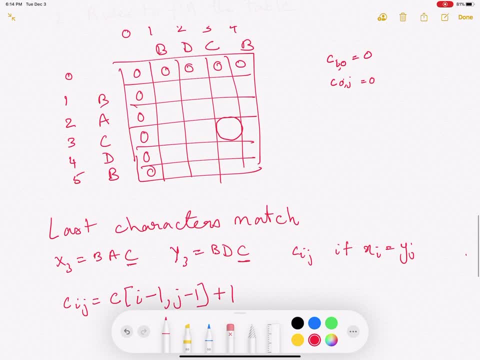 So, just to understand, when you're trying to fill this circle here, okay, what you know is you know these places already, Everything before it has been filled. So either we will move across in the row or we will move across the column. 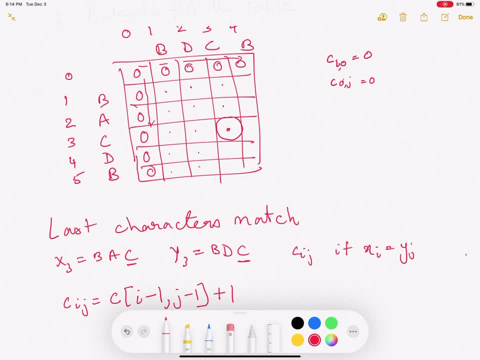 But if you move across rows as well, you would have filled it. So these positions would have been filled, most of them. So when you're trying to fill that- a bunch of things before that is known. So if you're trying to fill by columns, right. 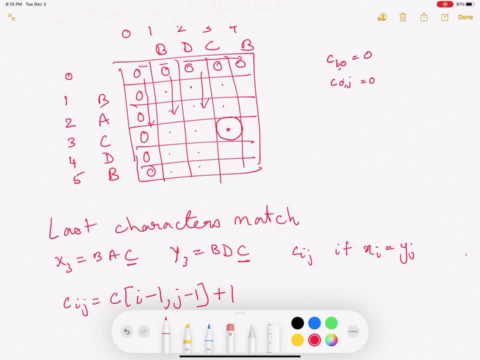 So we go, move along this column, then we'll move along this column. we'll move along this column, then we'll move along here. So this has already been filled, these places okay. So when you're trying to look at Ci-J- 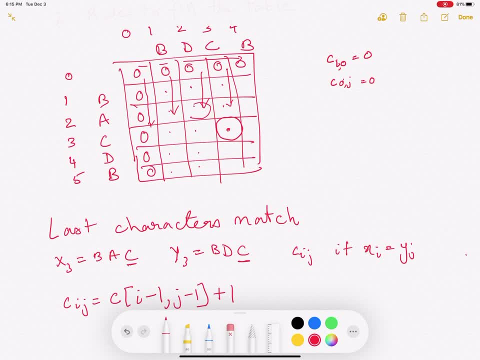 you already know what value exists in this block, So some value for the longest common subsequence exists. So to get Ci-J, what you're going to do is you're going to get see I-1, J-1, this is how I've written it. 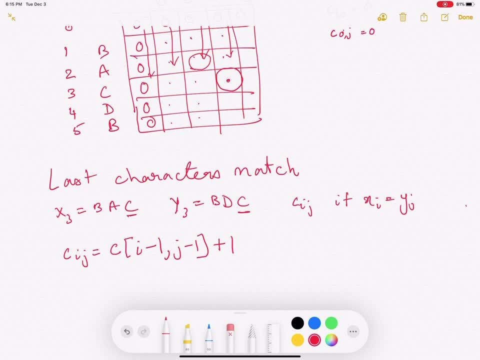 You can and you're going to add 1 to it. okay, So you're going to add 1 to it and add that. So, whatever entry is here, you're going to take that and do plus 1 to it, okay. 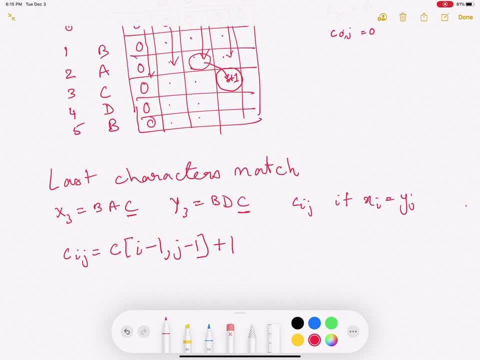 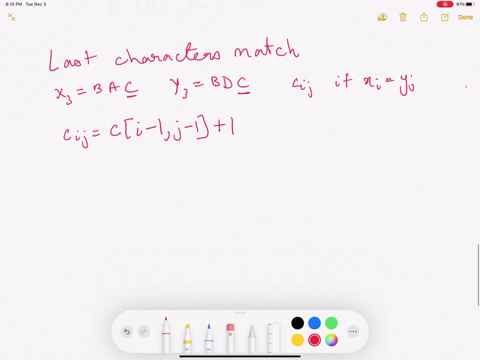 That is what will happen when last characters match, Okay, So the next scenario occurs when the last characters do not match. okay, So let's look at that condition. Last characters do not match, So we considered the case where the last characters match. 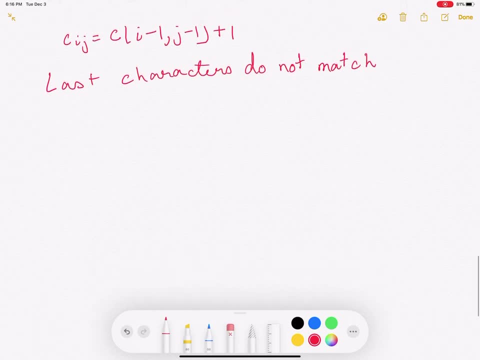 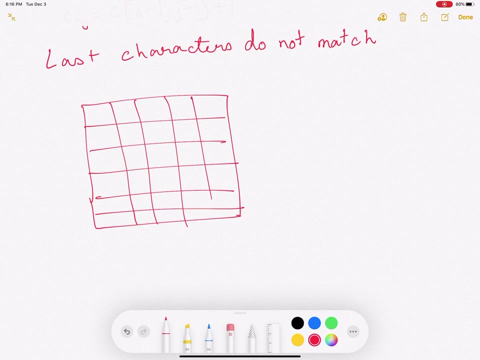 Now we are considering the case where the last characters do not match. When the last characters do not match, let's once again draw the table for our convenience. So we have the two strings as B-A-C-D-B. So we have the two strings as B-A-C-D-B. 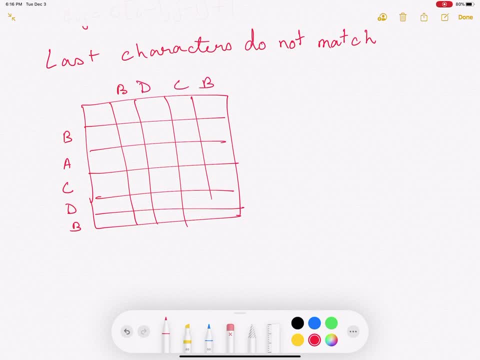 So we have the two strings as B-A-C-D-B. So we have the two strings as B-D-C-B, And this is 0, 1, 2, 3, 4.. This is 0, 1, 2, 3, 4, 5.. 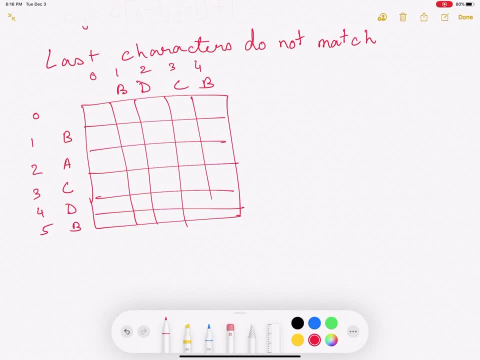 So the last characters do not match. Now, when we are trying to fill this block, okay, So the last characters don't match. So let's consider that we were trying to fill this. So we are looking at x. i equals to B-A-C. 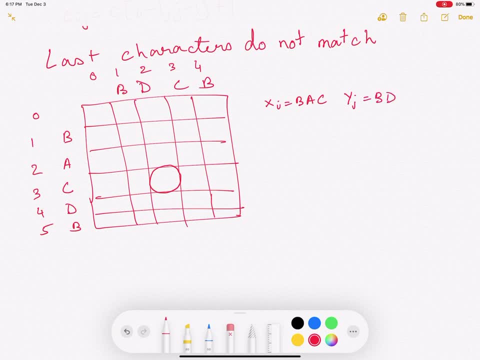 and y j equals B-D. okay, So we're comparing between those two. So the last characters do not match. Now, when the last characters do not match, one thing that we can be sure of is that both the C and the D. 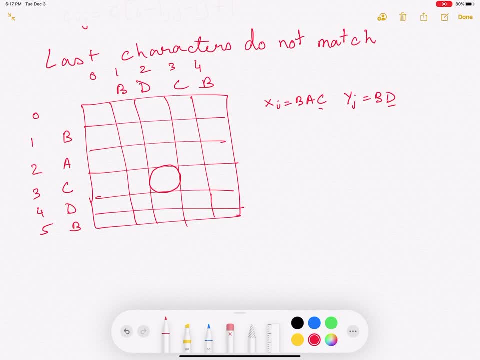 the C here and the D here cannot be part of the longest common subsequence, So both of them cannot be part. So what we can do is either we can try to find the longest common subsequence between BA and BD, which is this block here. 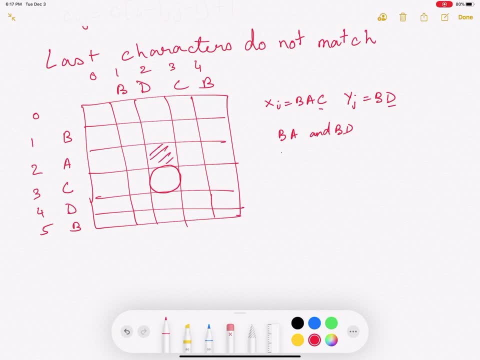 or we can look at BAC and B, because both of them cannot be part. So when you're trying to fill this, you already know that these blocks have been filled. They look here or here Now the CIG that we're trying to fill. 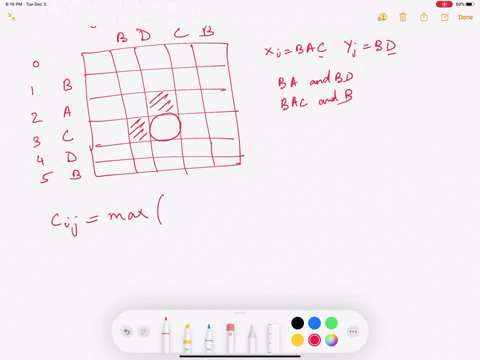 will be the max of C of I minus 1 J or C of I comma J minus 1.. So we'll look at this value here and this value here. Whichever is the largest, we will just take that and put it in here. 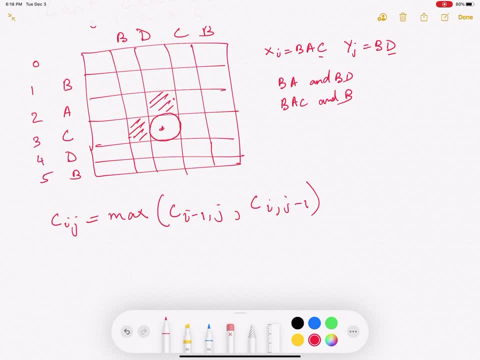 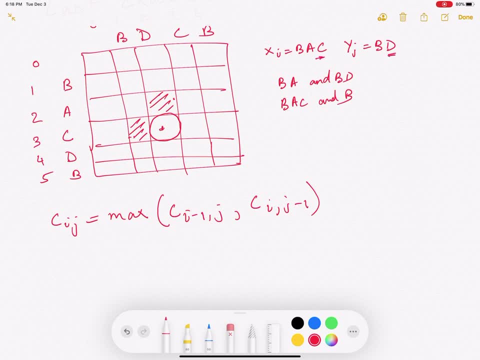 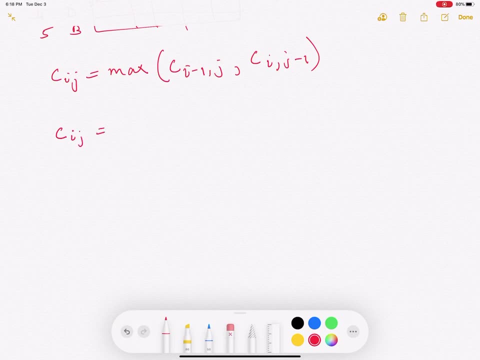 and D and D do not match, so both cannot be part. So whatever was the value earlier, that's what we put here. So, considering all this, what we get down here is CIG J. simple will be 0,. 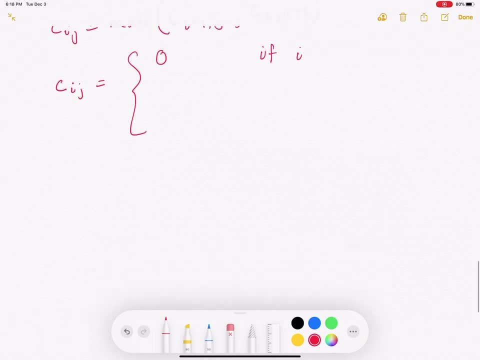 if this is the initial case, that is, if I equals 0, or J equals 0.. Okay, that's a simple case. That's the initialization. It'll be C, I minus 1, comma J minus 1,. 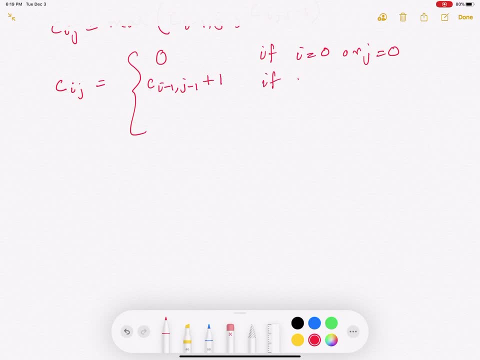 plus 1, if I and J are both greater than 0, and XI equals YJ, And it'll be equal to max of CI J minus 1, and CI minus 1, J if I and J are both greater than 0,. 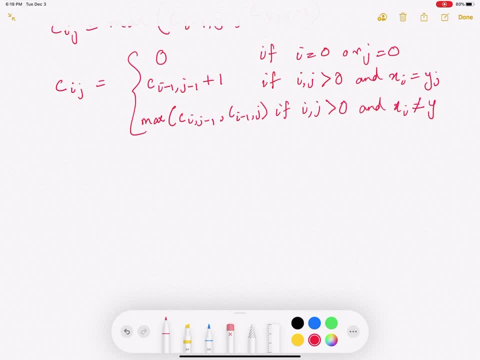 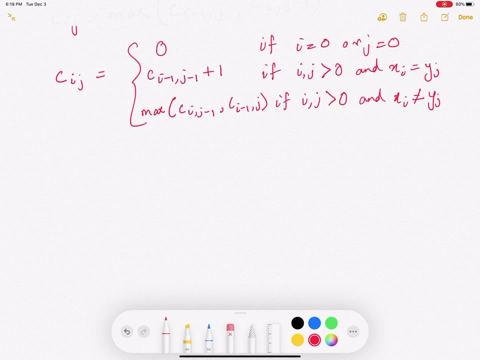 and XI not equal equal to YJ. That is the case. Okay, So this: these are the rules that we'll use to fill the table. Okay, So, so far, a lot of the stuff that we've covered is how we go about filling the table. 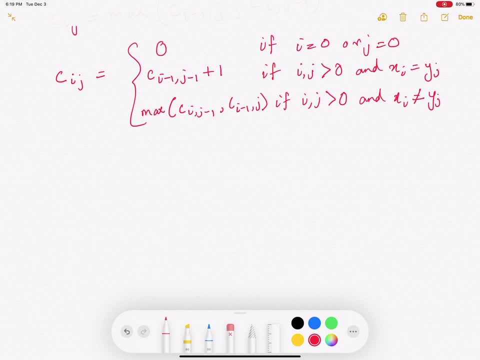 If you understand this, then you will be able to fill the table. So, basically, when you implement this using code, you will basically code up this portion, these equations, Okay, And that will help you fill up the table. Okay, Now that we have realized this. 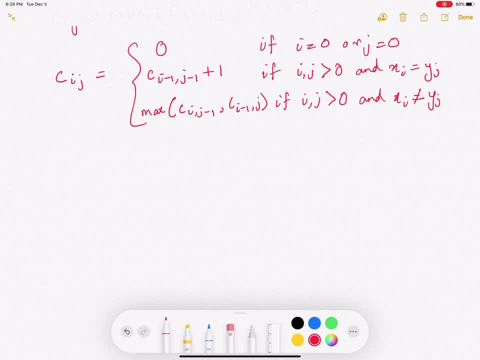 let's go ahead and draw the table again. See how we can fill this up. Okay So, with these equations here, Okay So, we have once again B A, C, D B here, And we have B D, C, D, B here. 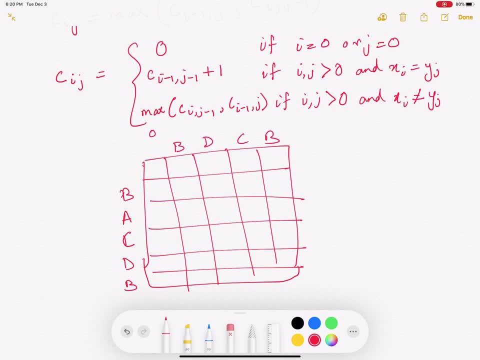 D, C, B, 0,, 1,, 2,, 3,, 4, and we have 0,, 1,, 2,, 3,, 4,, 5.. Okay, And if I or J is 0,? 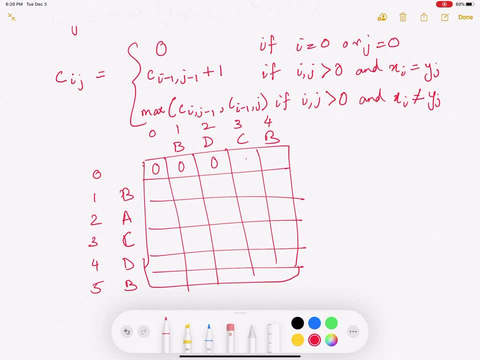 we are going to get all 0s in here, So we can put 0s here. Note that this table. at this point we have only talked about how to get the length of the longest common subsequence. Okay, But soon we'll talk about how we can actually 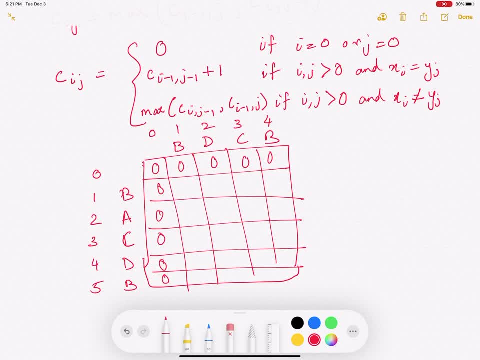 get the longest common subsequence as well. Okay, So now, once you fill this right, let's try to fill this block out here. Let's go by columns and go here. Let's just try to fill this block. We're going to try to fill that block. 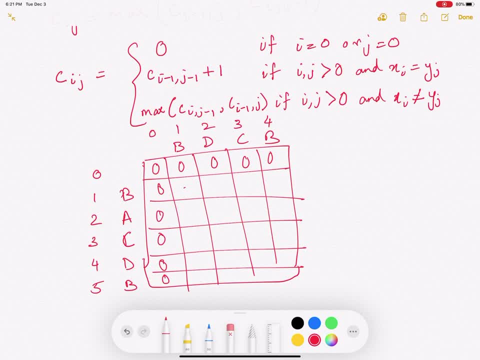 What do we get? We have? we're looking at B and B, Looking at two strings: X1 equal to B and Y1 equal to B. Okay, Okay, So those two strings have this last character to be the same. So we are going to look at the case. 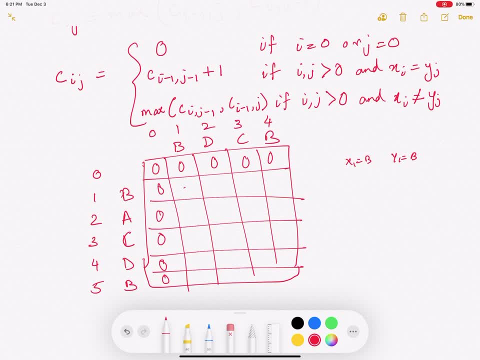 where the last characters are the same, which is basically I'm just going to write 1,, 2, and 3.. So we are going to look at case 2.. Okay, So we are going to add 1 to CI minus 1,. 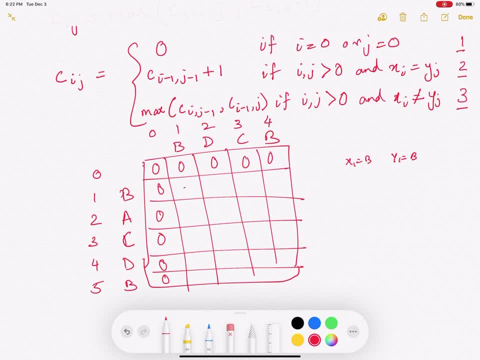 JI, So CI. here we are: I is 1, I equals 1, J equals 1.. So CI minus 1, J minus 1 will give us 0s. Okay, So we're going to do C11 will be C00 plus 1.. 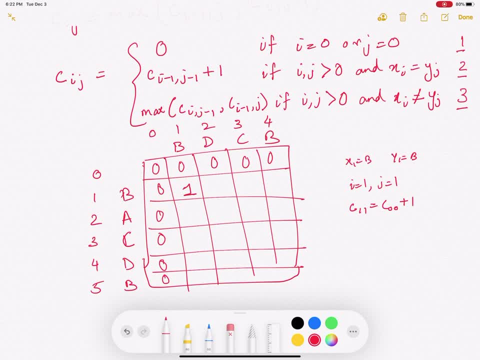 So you put a 1 in here. At this stage we are also going to keep track of some pointers. The pointer will tell you which box this value came from. So essentially, this 1 was filled using the 0 here. 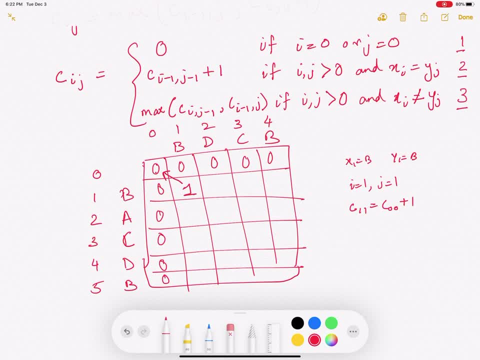 And that's why we are going to get that pointer there. Okay, Now if you, whenever you, when you, we may want to fill this value, Let's just try to fill this one. Okay, You can go either by row or by column. 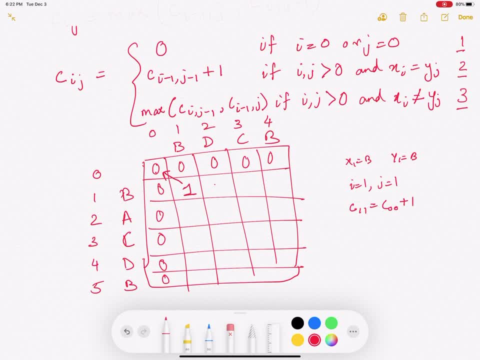 It does not matter. Okay, So we want to fill that. Now we are looking at X1,, B and Y2, which is basically BD, And we get to the case where the last characters, that is, B in this case, and D. 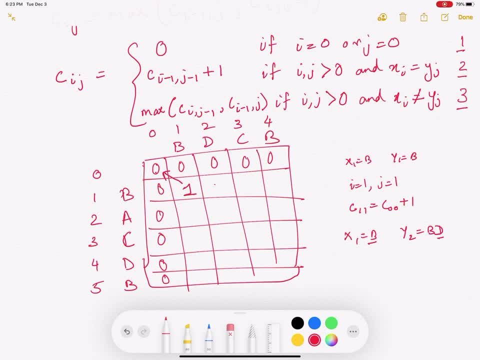 they do not match. Therefore, what are we going to do? We are going to look at this column and this column and this, these two boxes- not the columns, but these two boxes- And you're going to take the max, which is essentially max of 1 and 0,. 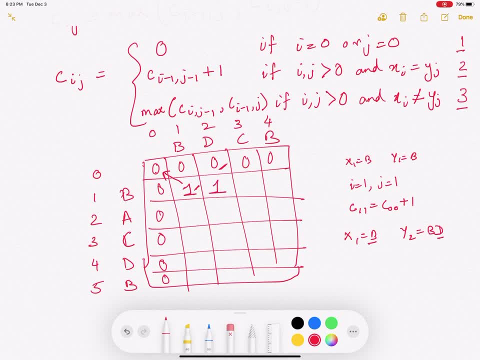 which is 1.. So we're going to put a 1 out here and you're going to put an arrow here. Okay, Just going to take this eraser and erase this, So we put a 1 there. Now you can try to fill this one against the. 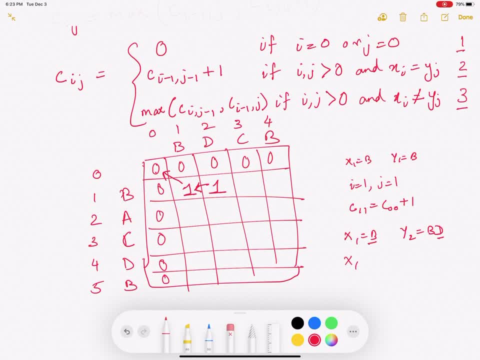 it'll be basically between X1 equals B and Y2 equals BDC. Again, the characters don't match. So you will look in this box and in this box 1 and 0, compare that of course 1 is greater than 0.. 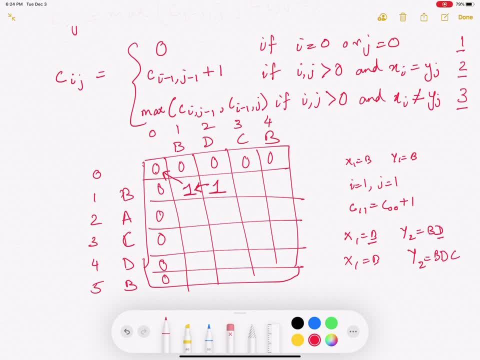 So you are going to take 1 out here, put an arrow Like this, And if you fill, you will get to the state. So I'm not, I'm just going to fill out these, these with the zeros as well. 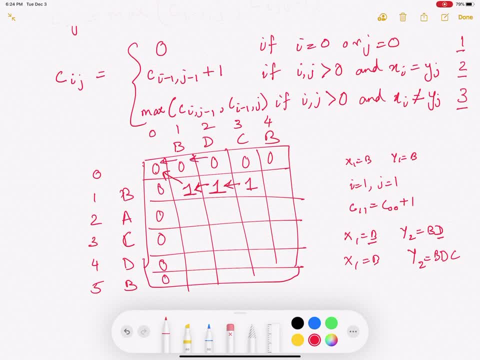 I'm just going to put the arrows so that it helps you understand. So this is how these arrows would be And if you just solve it, you will know that this is the direction of the arrows. I'm just going to do it for ease of understanding. 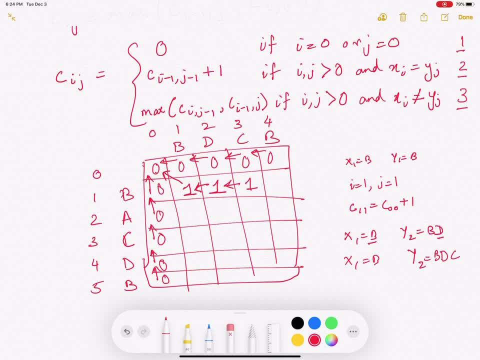 We'll look at another. Now let's look at this box. Okay, So this box, this is: X1 equals B, and X4, which is, and Y4, which is BDCB. So or sorry, it's BDCB. 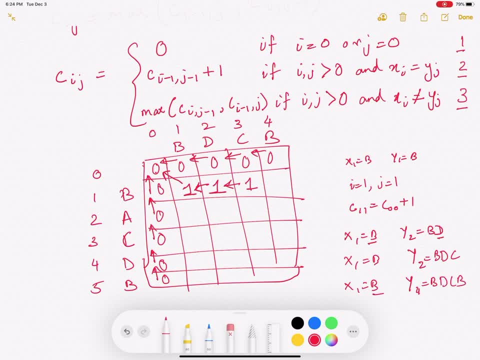 So it's going to be BDCB, So the last characters match. Therefore, you are going to look at this box, which is a 0, and add 1 to it, Okay, So, therefore, what are we going to do? 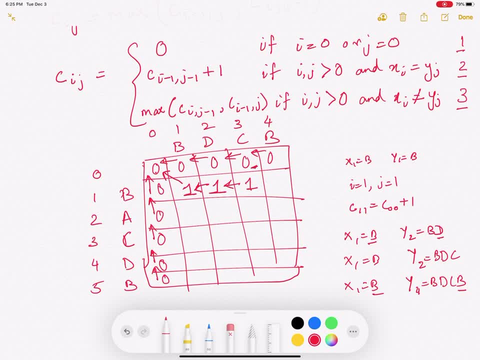 It's going to be 0, in this box here plus 1, which is going to be 1.. It is important where you get the 1 from, because you are going to use the pointer to keep track of that. I'm just going to erase the first. 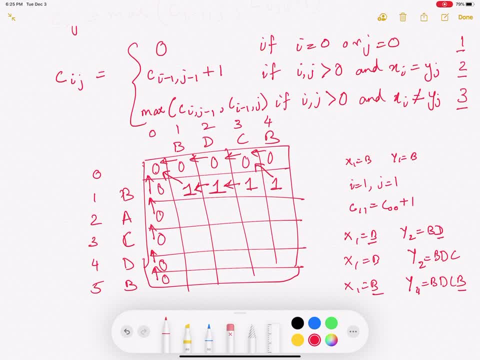 So you're going to put an arrow pointing out here. In this way, we can fill the rest. So I'm just going to fill a few of those. It's going to be a 1 here which is going to come out of here. 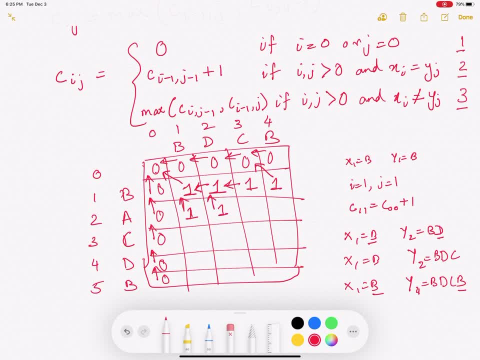 There is going to be a 1 here which is going to come out of here. There's going to be a 1 here which is going to come out of here. There's going to be a 1 here which is going to come out of here. 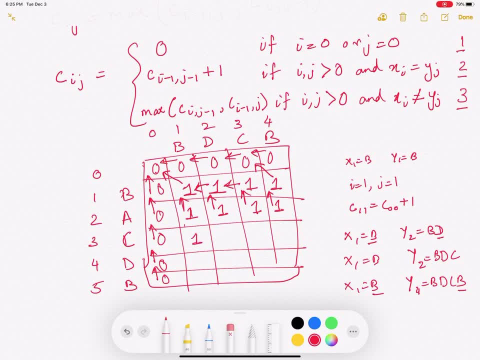 Okay, Similarly, you're going to have a 1, which comes out of here, Another 1, which comes out of here. Now, let's just consider this one. So this position. Now I'm just going to erase these things. 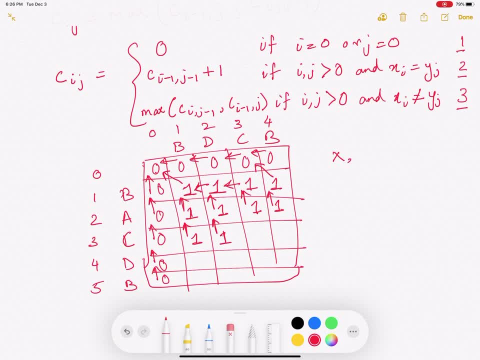 So we're looking at X3,, which is BAC, and Y3,, which is BDC. So we are at the case where the la characters match Okay. So we have to look when you're trying to fill this box, this box, out here. 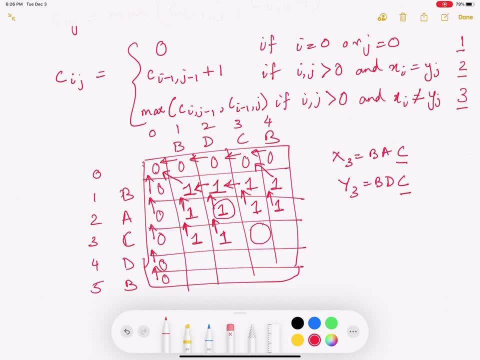 You look at this box. Okay, Because the characters match. So we're going to add 1 plus 1, which is going to give us 2.. so i'm just going to erase this and also the circle, so you will get two and there will be. 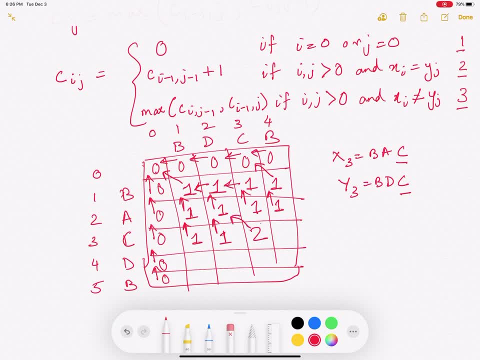 an arrow pointing out here the same. when you, if you look at this box out here, this one, that's the box that we're going to fill, then we will have. we're going to look at x3, that is bac and y4 that is b, or b, d, c, b. okay, now, let me just get rid of this now to fill that. the last characters they. 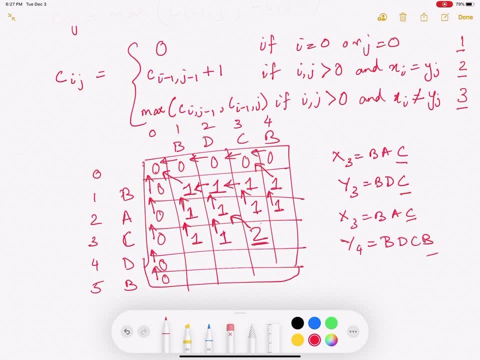 don't match. therefore, we are going to consider this box and this box, take the max and put it in there. okay, so once again, i'm going to erase the underlining. so we're going to between two and one. the max is two. you're going to put, put an arrow like this here: 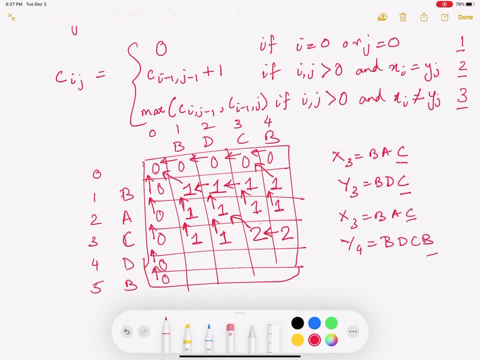 okay, now, in this way you can fill the rest of the table. i don't want to go on doing the same thing. so you will have one here, you can have a one here and you will. you will see that you will have a two here which actually comes from here and you will have another two which comes from here. 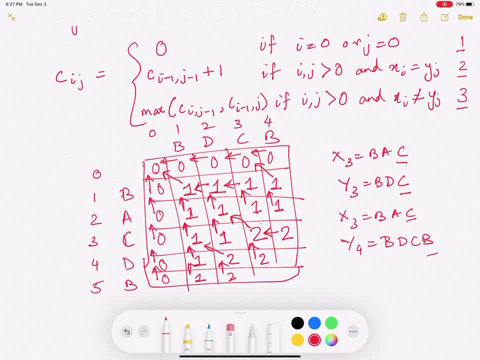 there will be a two here which comes from here, there will be another two here which comes from here, and there will be two here which comes from here. let's just fill the last box. so now i'm just going to take get rid of these this side. 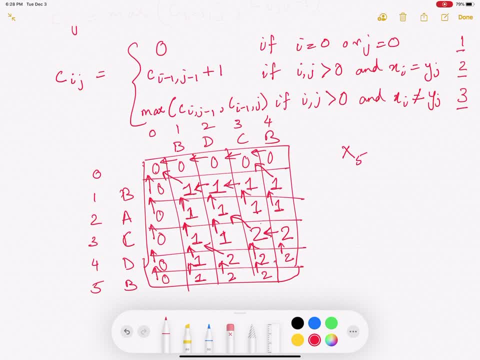 so what we are considering is x5, that is b a, c, d b, and y4, that is b d, c b. the last characters match here. so what we will do is, when we are trying to fill the x box, we're going to look out here. 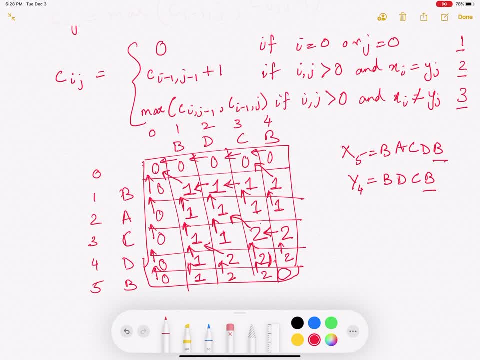 that box, okay, and you're going to add one to the two there. so i'm going to use the eraser to get rid of these, this one, and so what you're going to get here is 2 plus 1, that is 3. so you're going to get a 3 here and this. 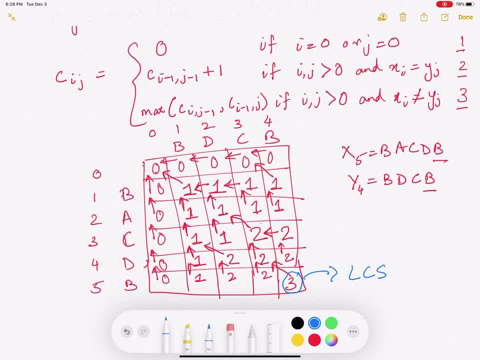 is your llc, so what you're going to get here is 2 plus 1, that is 3. so you're going to get a 3 here. and this is your llc, so what you're going to get here is 2 plus 1, that is 3. so you're going to get a 3 here. 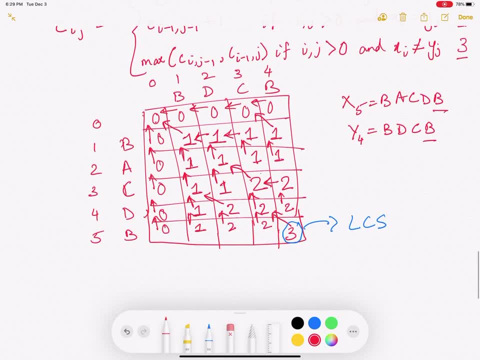 and this is your llc. so what you're going to get here is 2 plus 1, that is 3. so you're going to get a 3 here and this is your llc. so you're going to get a 3 here and this is your llc. so you're going. 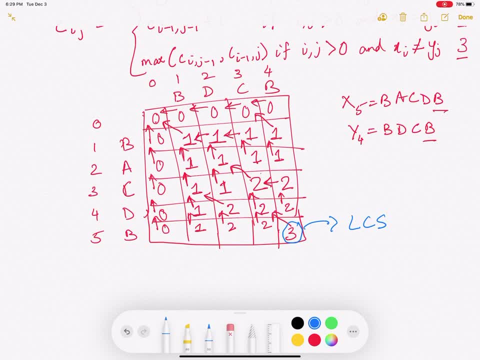 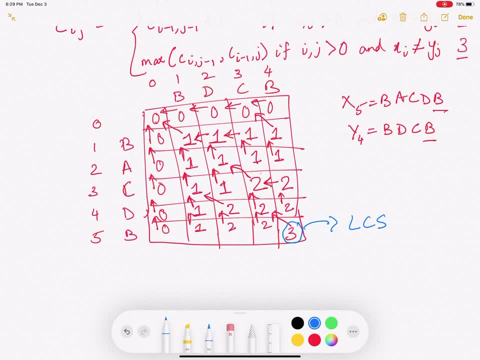 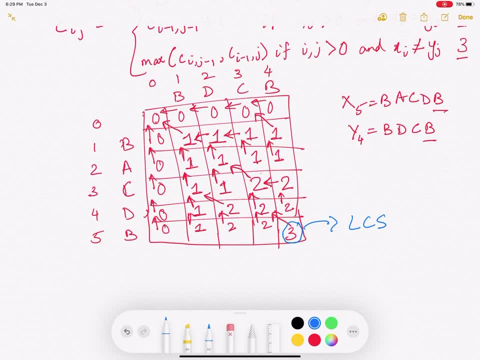 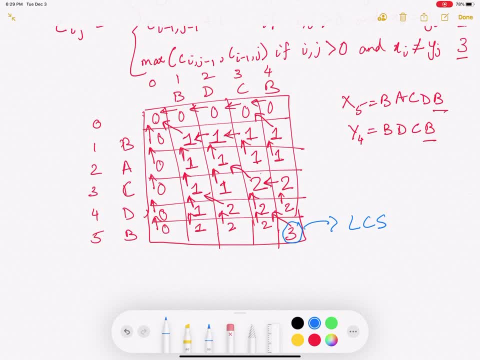 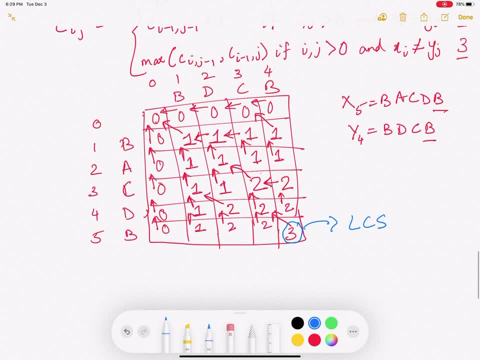 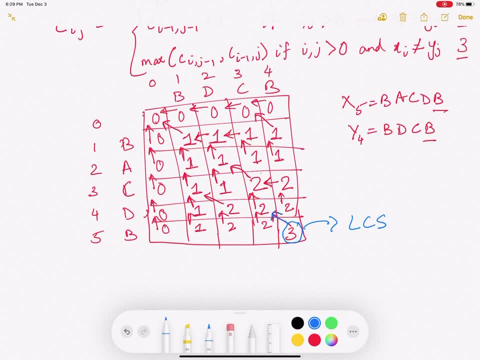 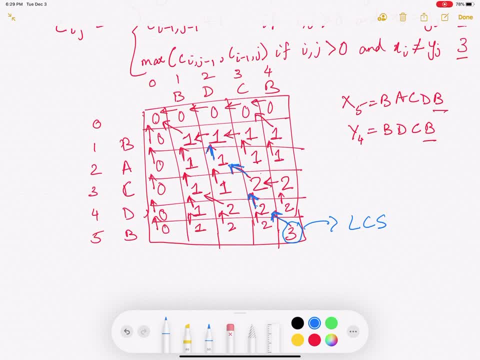 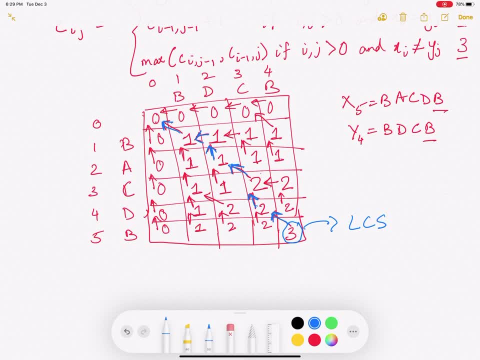 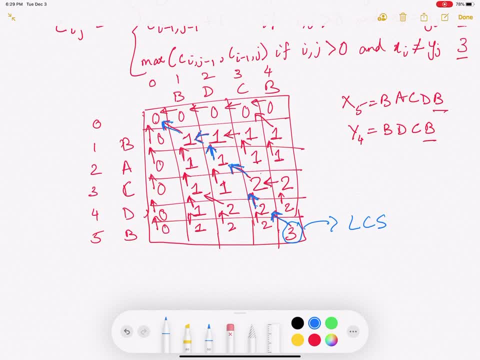 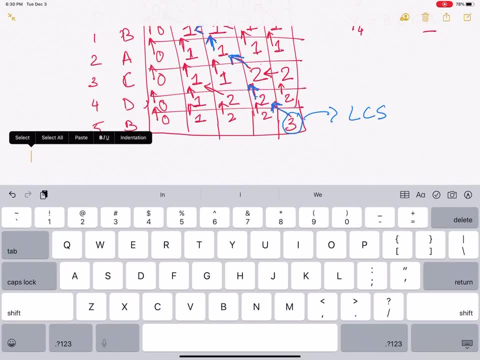 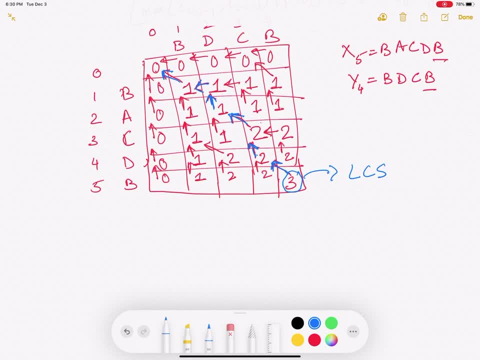 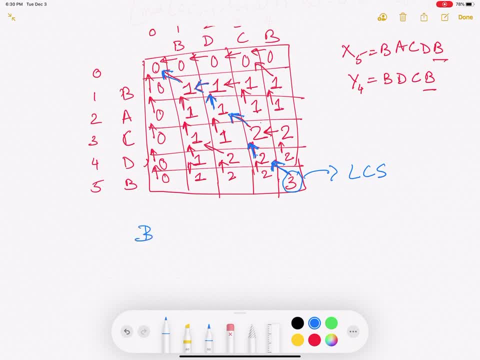 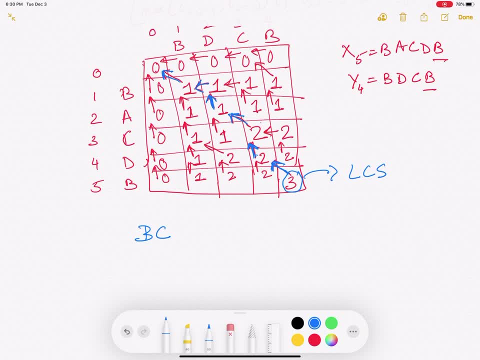 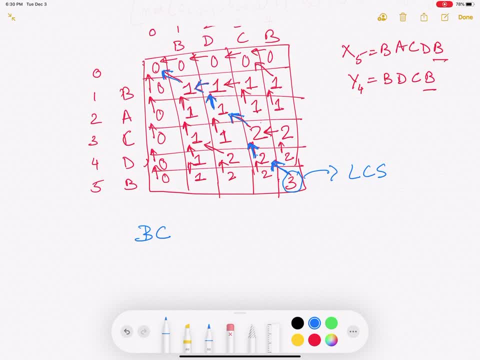 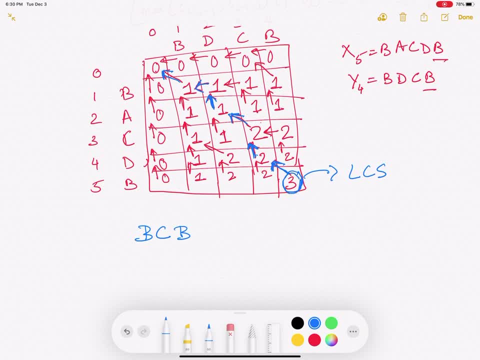 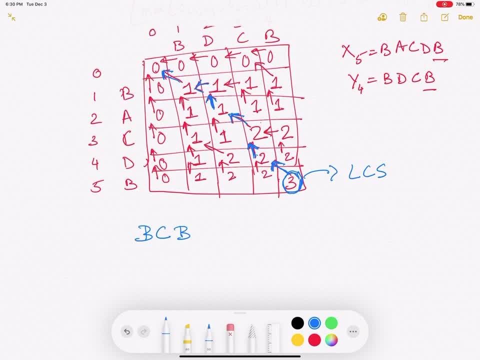 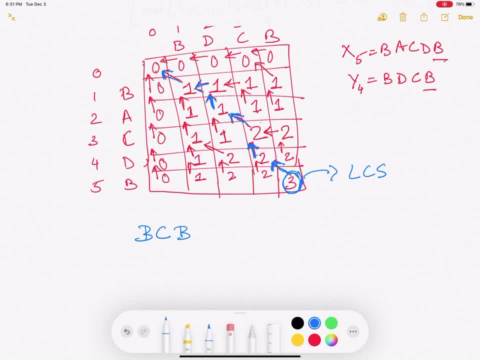 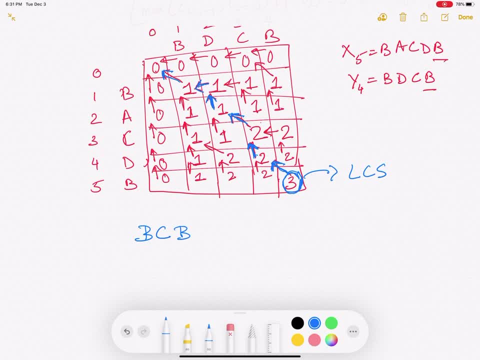 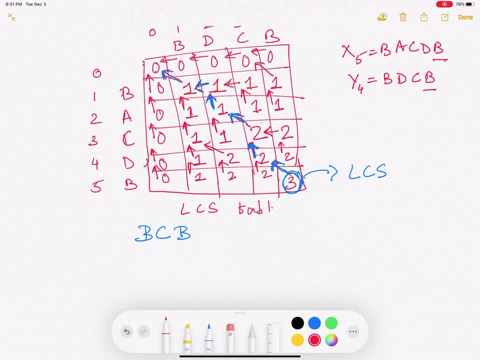 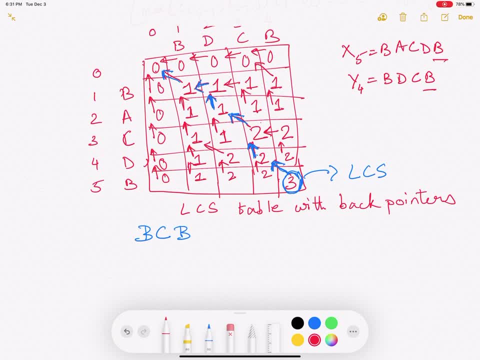 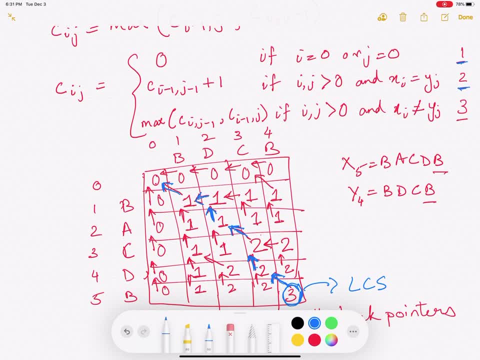 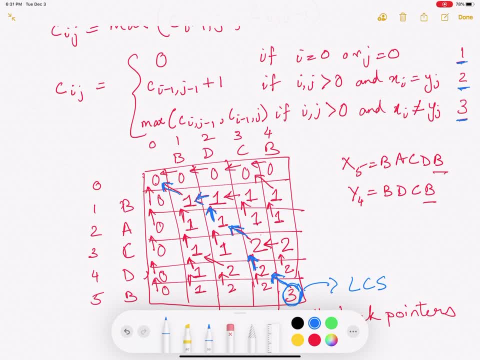